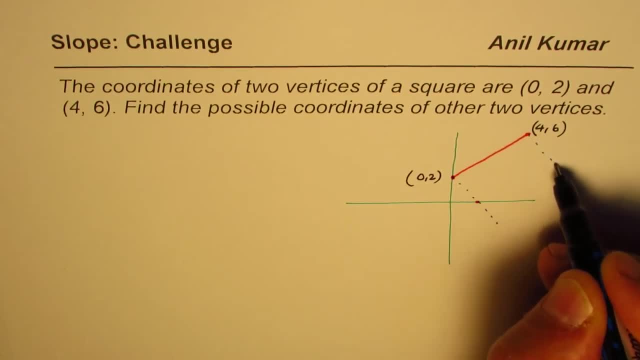 this: Do you see that? Which will be right angle, So that could be one possible square, correct? So we could make something like this. Or we could also make one square on the other side, right, So you could also make a square on this side of this line, correct? So? 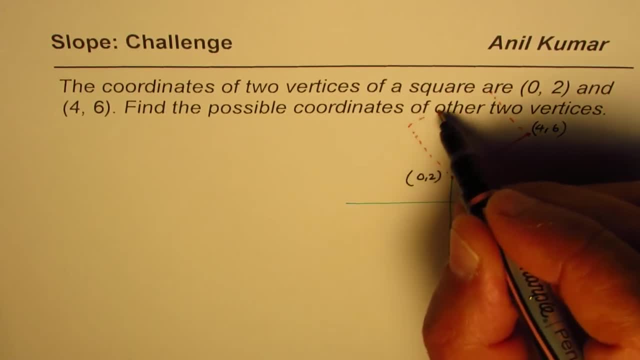 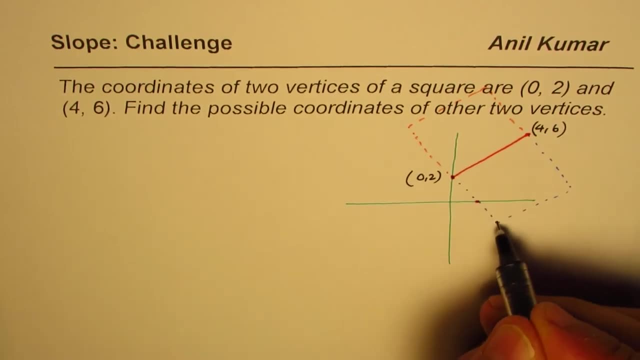 we could also make something like this. So these are definitely two possible situations. Now, how to find the coordinates of these points, That is the question for you. So I hope you have understood, So you can pause the video and answer the question. 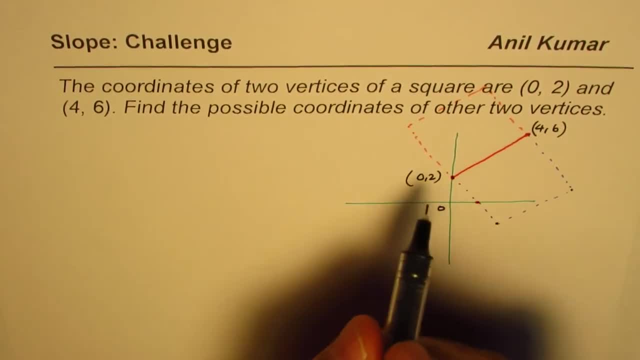 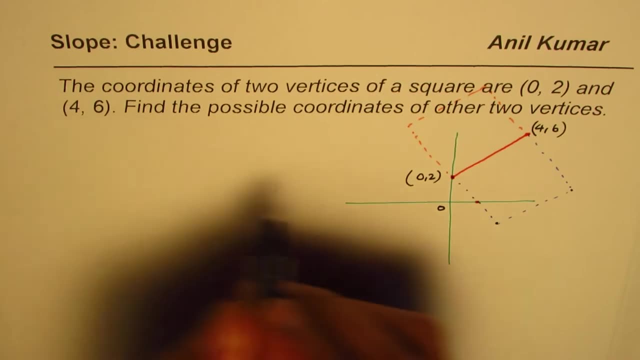 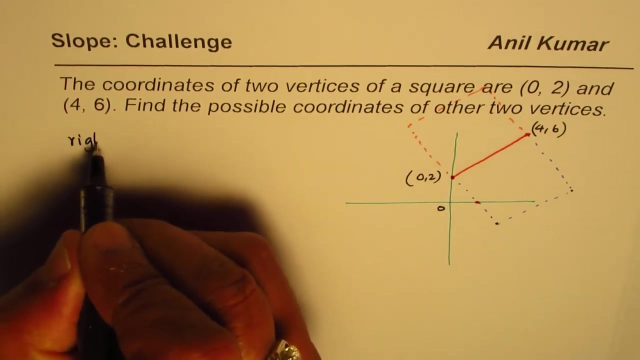 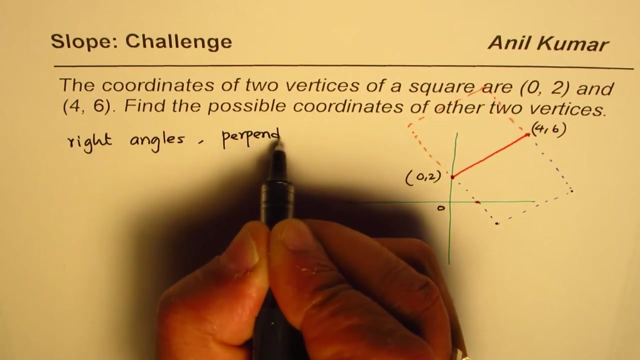 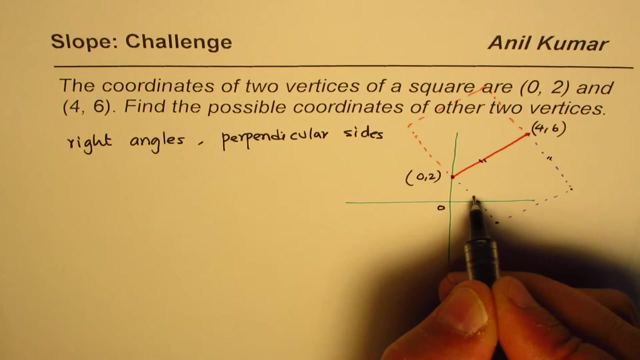 Now the strategy here is the slope of the other side, adjacent side, will be negative, reciprocal of this slope right. So we know the corners are right angles, So we have right angles or perpendicular sides. This is one thing Plus. we also know that all sides are equal in length. 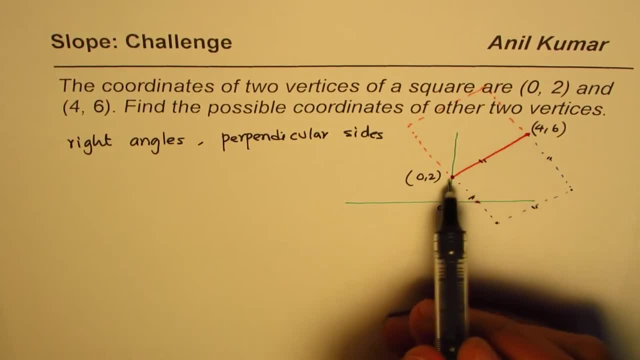 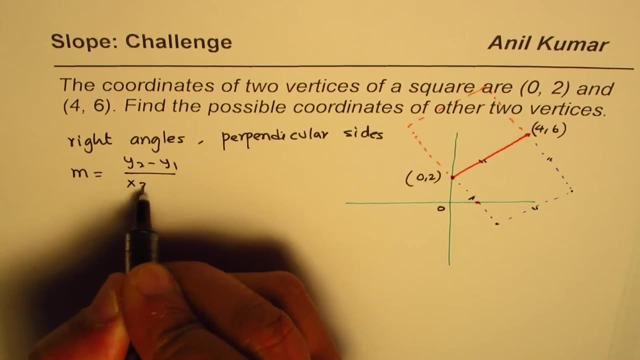 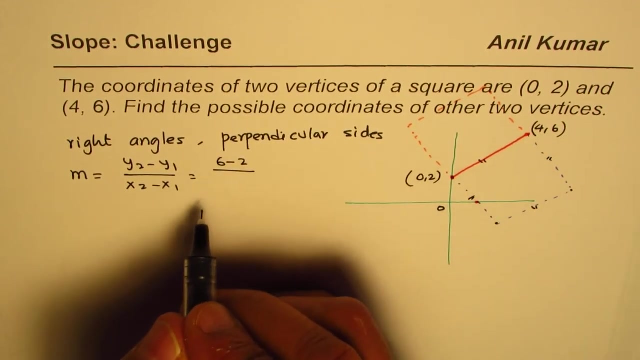 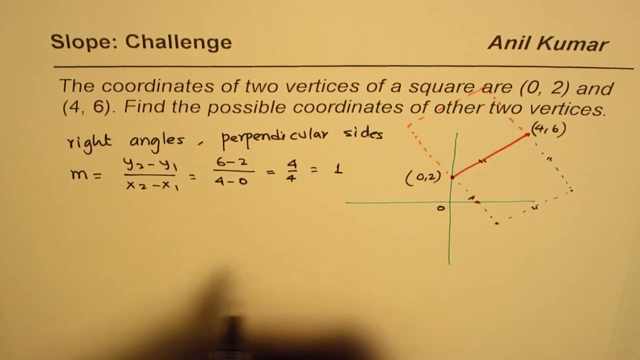 right Now let us find the slope of the segment given to us. Slope M will be y2 minus y1 divided by x2 minus x1, 6 minus 2 divided by 4 minus 0. That gives us 4 over 4, slope of 1.. Now 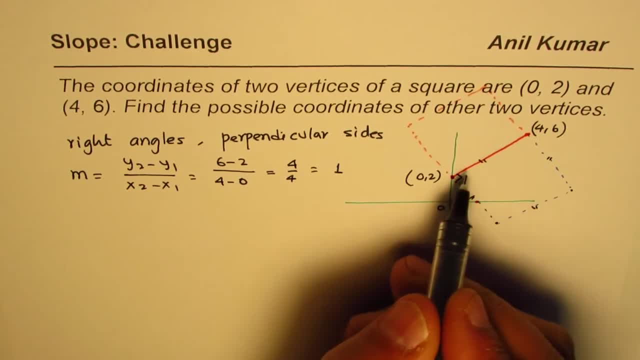 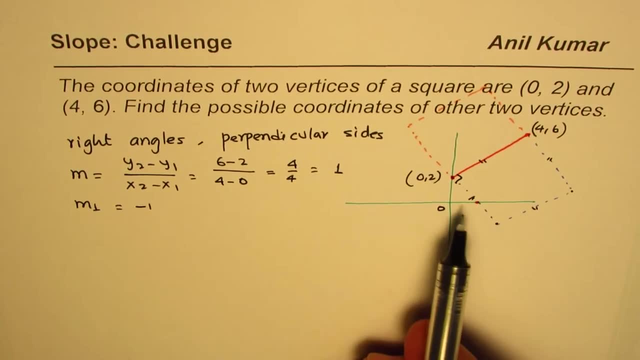 this line, which is perpendicular to the given segment, will have a slope of negative 1, right, negative 1.. So we know that the slope is going to be negative 1.. Now, as you see here, when we say slope of 1, if I move from point, let us say point A to: 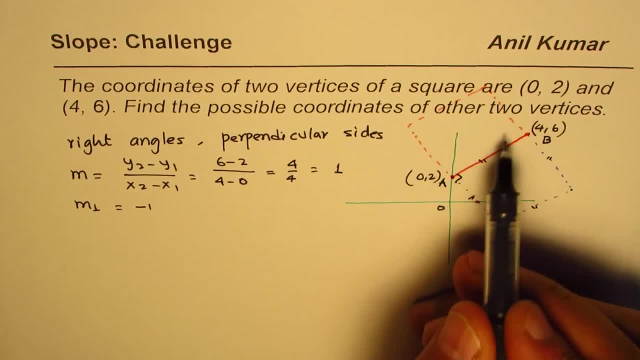 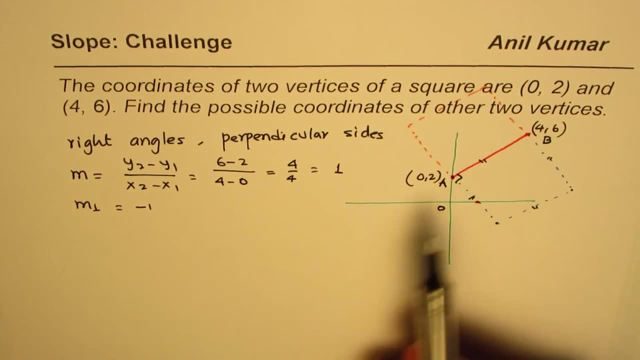 point B: I am going up by 4 and right by 4, right, So that is the movement. So when I have a slope of minus 1, I can go up by 4 and right by 4, right, So that is the movement. So when I have a slope, 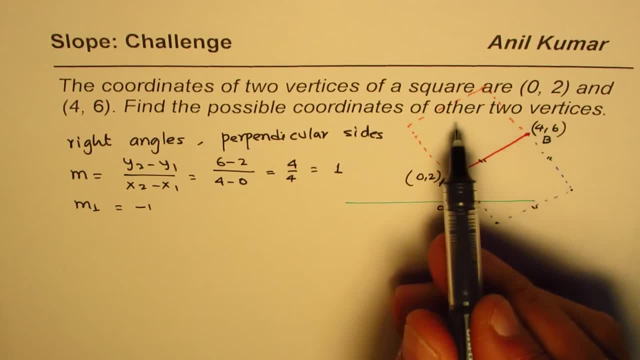 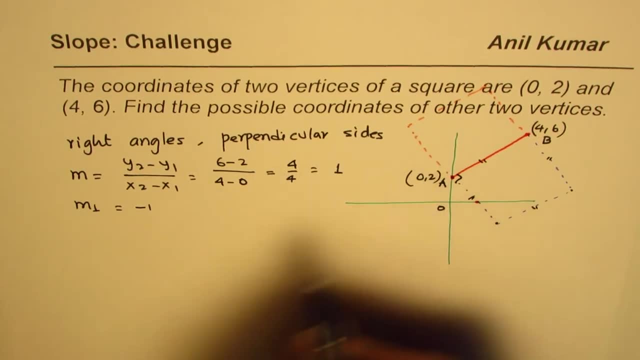 of minus 1, I can go up by 4 and right by 4, right, and instead of moving right we can move left by 4.. So if I do that, we get negative slope right. So what we will do here is beginning from 0,. 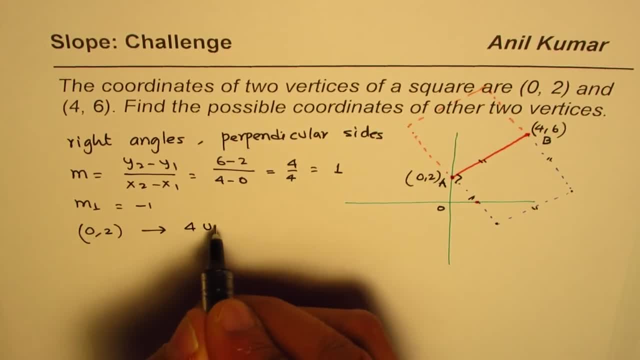 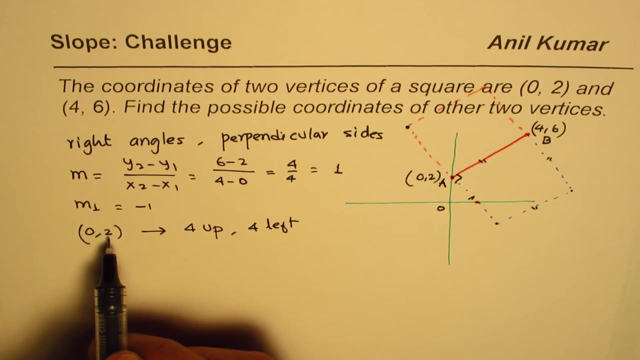 2, we will move 4 up right, 4 up and 4 left. So if we do that, where will we reach? We will reach at one of the points of this square. Four up means the y value increases by 4.. 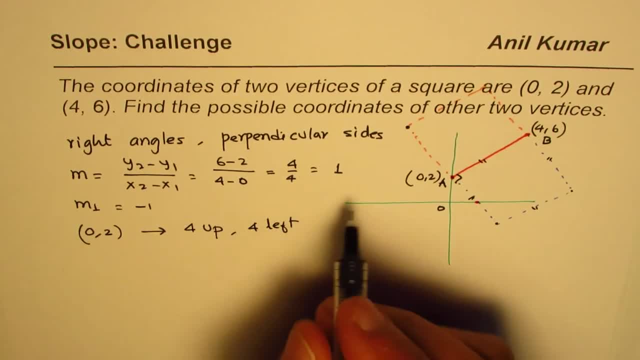 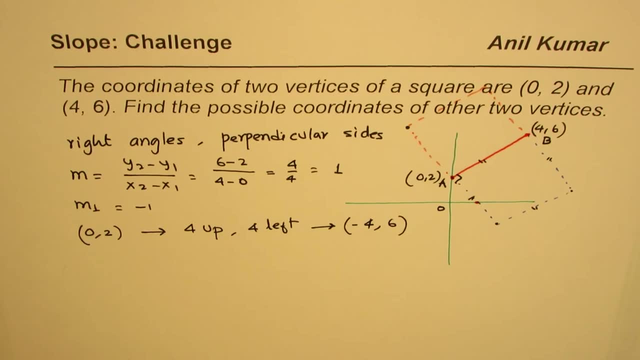 4.. 4 left means x, value decreases by 4.. So that will give us minus 4, and 4 plus 2 is 6 as this coordinate. Do you see that point? Same thing will apply to the second point, which is 4, 6, right. 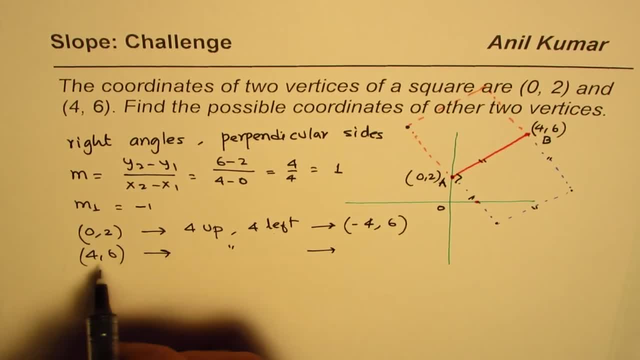 So we are going 4 up and 4 left. So up means add 4 to 6, which is 10, and left means take away 4 from 4, which is 0.. So one set of points, are these right? So these are one set of points. 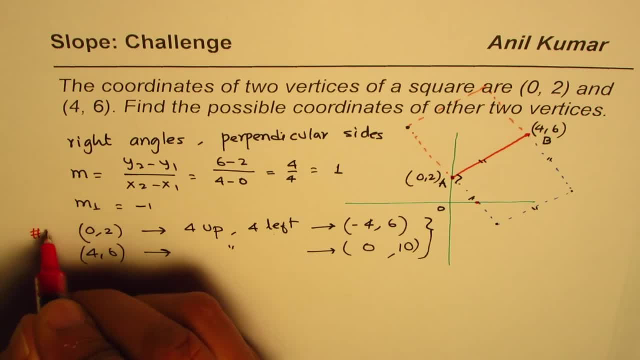 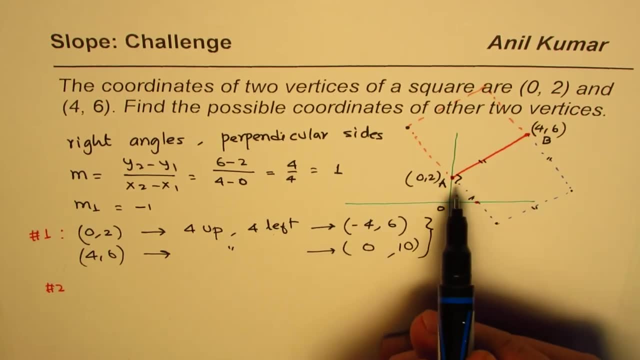 So that is one solution, right. So we have set 1, right, Now let us do set 2.. To find the second set of points, we can move this time 4 down and 4 right. Earlier we were going. 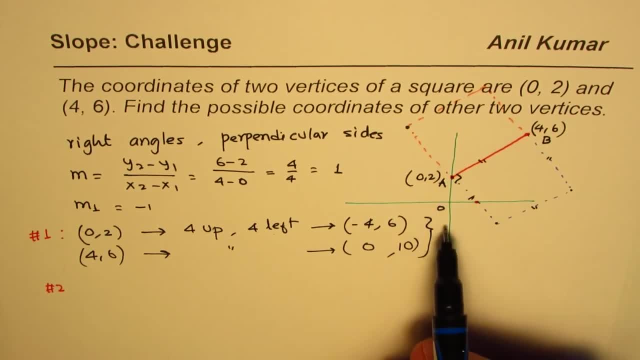 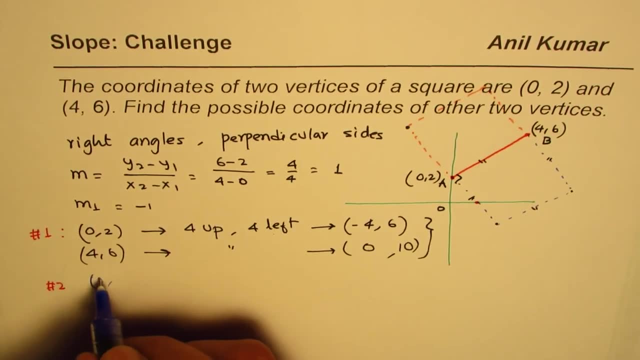 4 up and 4 right. Now we should go 4 up and 4 right. So we are going 4 up and 4 right. So, starting with 0, 2, we need to go 4 down- Let me write down- and 4 right. That really means that. 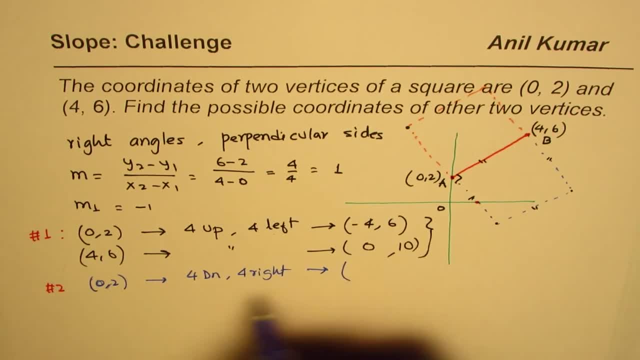 the y value will be decreased by 4.. So 2 minus 4 is minus 2.. 4 right means add 4 to x value. right, Starting with the point 4, 6, 4 down, and 4 right means y value decreased by 4.. 6 minus 4 is 2 and the x value increased by. 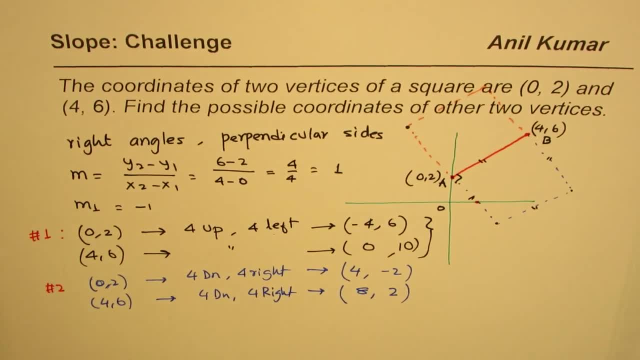 4. We get 8, correct, So that becomes the second set of points. So now we can write down our answer, as the coordinates could be minus 4, 6 and 0, 10, or the second set could be 4 minus 2 and 8, 2.. So that is how you can actually. 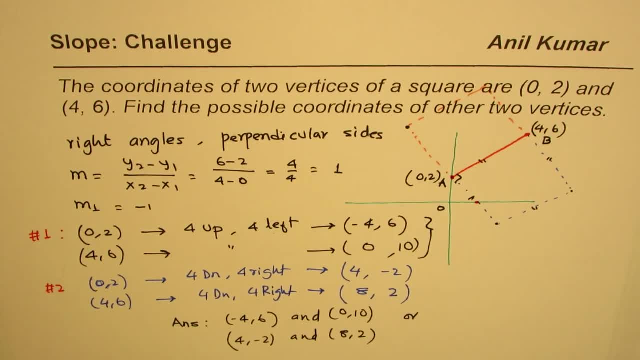 answer this question. I hope that helps. Thank you and all the best.